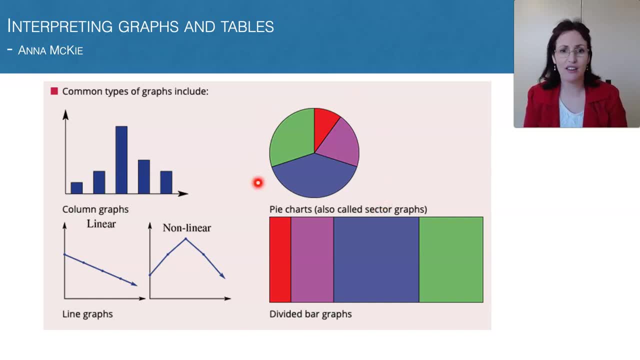 or a pie graph, sometimes sector graphs, And the whole thing represents 100%. We might have a divided bar graph here And then these are both called line graphs because they both involve straight lines, But this one we call a linear graph. Notice that the word linear has line in it And the difference. 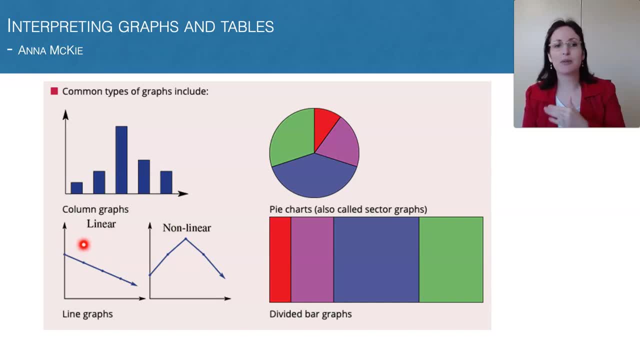 between these two. technically, what's happening here is the rate of change between all of the points on the graph is the same. So this is a true linear graph And this one. here, although there's straight line sections, they change from time to time, So we call that one non-linear. 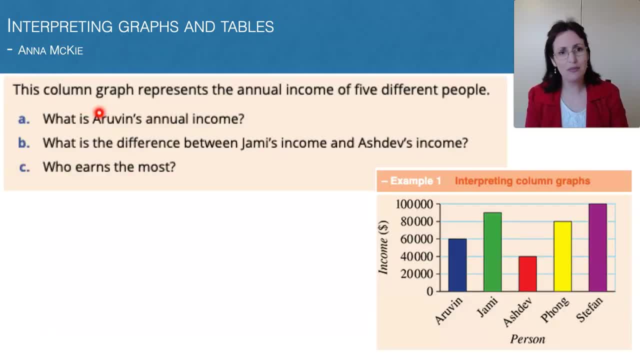 So these questions. First one: the column graph represents the annual income of five different columns, And this graph represents the annual income of five different columns And this different people. let's take a moment just to look at the graph that we're asked to describe on our 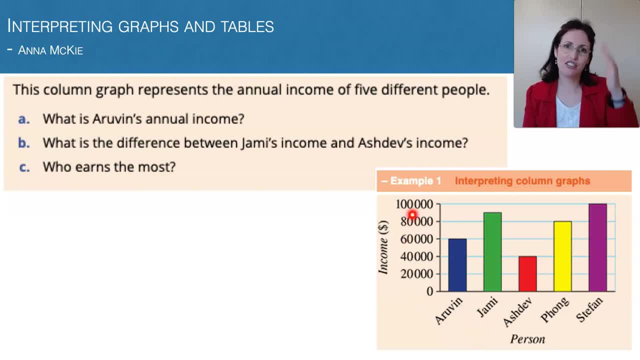 horizontal axis we've got five people and on the vertical y-axis we have their income in dollars. notice that that's going up in twenty thousand dollars each time part a what is a Reuven's annual income? let's find a Reuven on the graph. that's the blue column. we read up to the top of the blue. 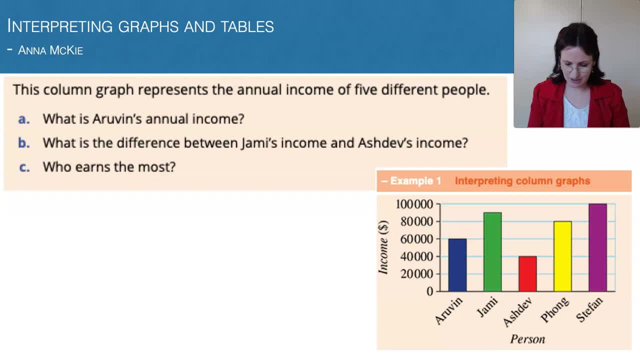 column across to the vertical y-axis and we have sixty thousand dollars. so for what is a Reuven's annual income we would write sixty thousand dollars. I have put that little comma in there. sometimes we do that in maths to separate groups of three numbers. but you don't have to. 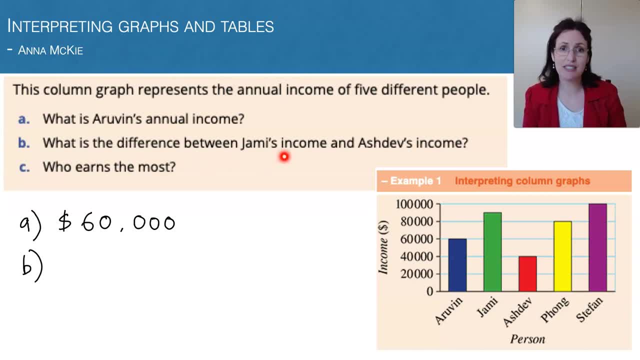 part b: what is the difference between Jamie's income and ashdev's income. so let's have a look over here first, where is Jamie? that's the tall green column and ashdev, the shorter red column. and what is mean in maths? what operation do we need to do a subtract, so you need to do the biggest number. 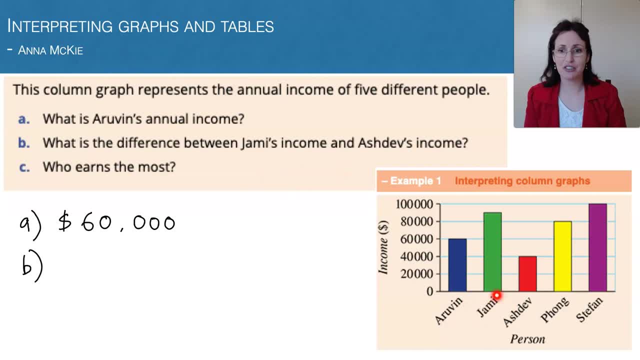 subtract the smallest number which is the biggest number out of these two, the green one. so let's read up and see how much that is. it's between the two blue lines. we're assuming it's about halfway between. so halfway between 80 and 100 000 would be 90 000 for jamie. so what's the difference between? 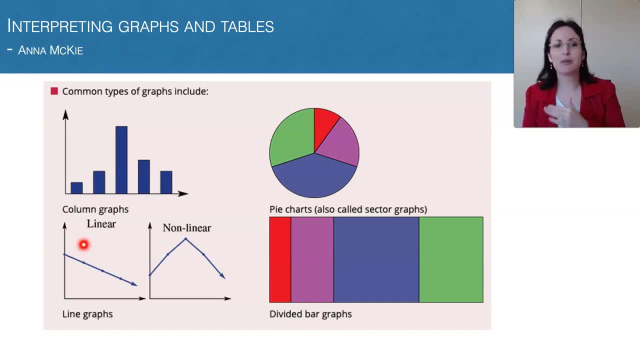 between these two. technically, what's happening here is the rate of change between all of the points on the graph is the same. So this is a true linear graph And this one. here, although there's straight line sections, they change from time to time, So we call that one non-linear. 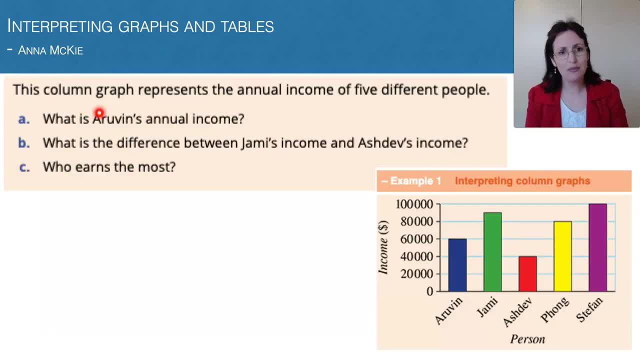 So there are these questions. First one: the column graph represents the annual income of five different people. let's take a moment just to look at the graph that we're asked to describe. on our horizontal axis we've got five people and on the vertical, y-axis, we have their income in dollars. 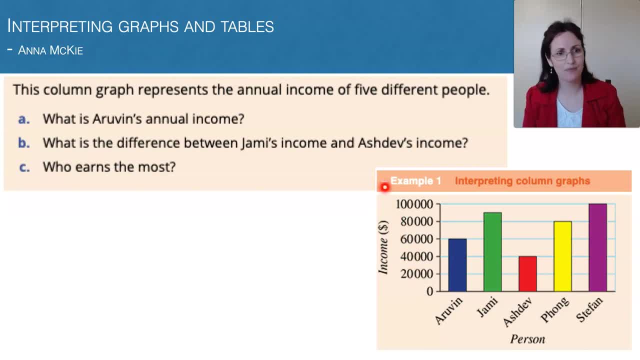 notice that that's going up in twenty thousand dollars each time part a. what is a Reuven's annual income? let's find a Reuven on the graph. that's the blue column. we read up to the top of the blue column, across to the vertical y-axis, and we have sixty thousand dollars. so for what is a? 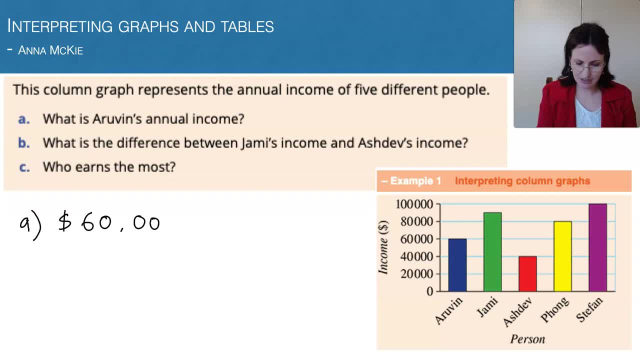 Reuven's annual income, we would write sixty thousand dollars. I have put that little comma in there. sometimes we do that in maths to separate groups of three numbers, but you don't have to part b. what is the difference between Jamie's income and Ashdev's income? so let's have a look. 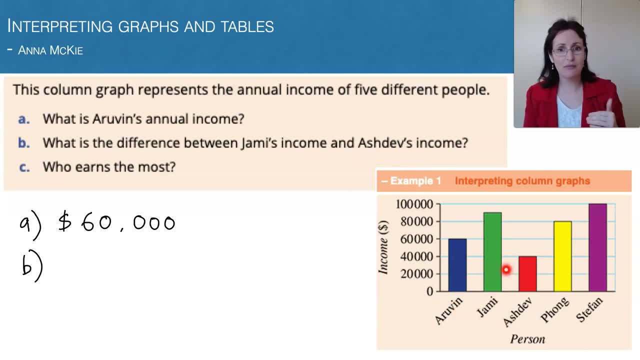 over here. first, where is Jamie? that's the tall green column, and Ashdev, the shorter red column. what does that mean? difference mean in maths? what operation do we need to do a subtract? so you need to do the biggest number subtract the smallest number. which is the biggest number out of these two, the green? 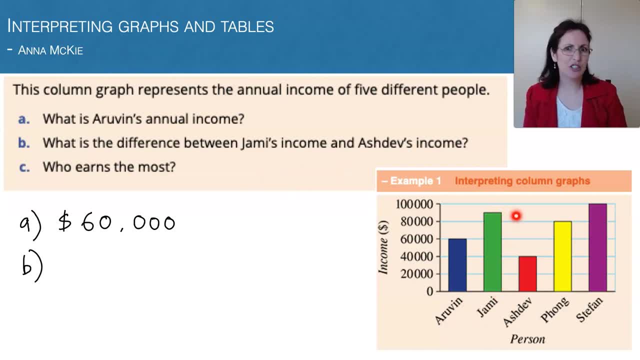 one. so let's read up and see how much that is. it's between the two blue lines. we're assuming it's about halfway between. so halfway between 80 and 100 000 would be 90 000 for Jamie. so what's the difference between Jamie and Ashdev's? ninety thousand dollars for Jamie, Ashdev reading up and 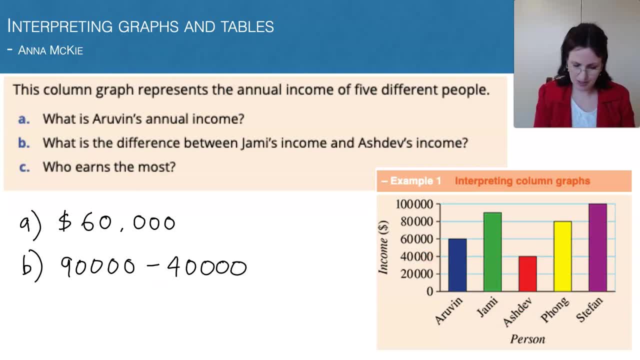 forty thousand dollars, and the difference between those two is fifty thousand. again, you can put the comma in or not, it doesn't matter. okay, who earns the most, who- we're after a person- and the most the tallest column over here, the purple column, is the tallest. and who does that belong to? Stefan or Stefan? 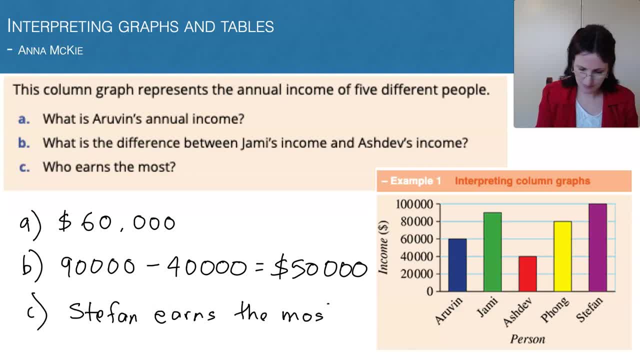 how does that answer the problem? what is the number six column for 접, PlayStation or Stefan? what does that rank? what is the number four column? I think it's good to create a column and I'll add this in here first. if you did a good job, so you'll. if you're going to ask a question, is this column for who? you crashed this Moving Fr? indulge opinion. 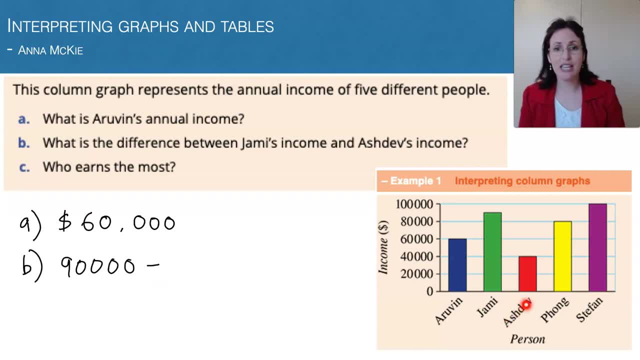 jamie and ash devs. ninety thousand dollars for jamie ashdev, reading up and across forty thousand dollars, and the difference between those two is fifty thousand. again, you can put the comma in or not, it doesn't matter. okay, who earns the most, who- we're after a person and the most? 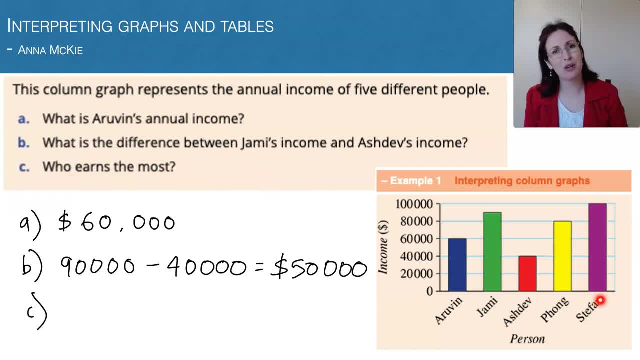 the tallest column over here, the purple column is the tallest, and who does that belong to? step? and or stefan? i think it's a good technique that when you're asked a question in a sentence, it's a good technique to practice writing the answer in a sentence. who earns the most? stefan earns the most. 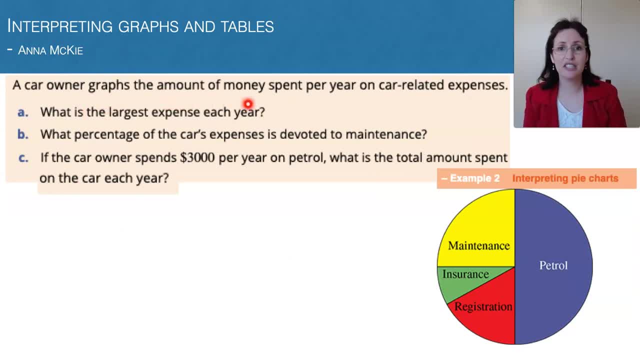 second question: a car owner graphs the amount of money spent per year on car related expenses. so let's have a look here of our pie chart. these are all the different costs that you might spend. um, if you are in a car, about that much is petrol. how much of the graph would you say that is half or 50? 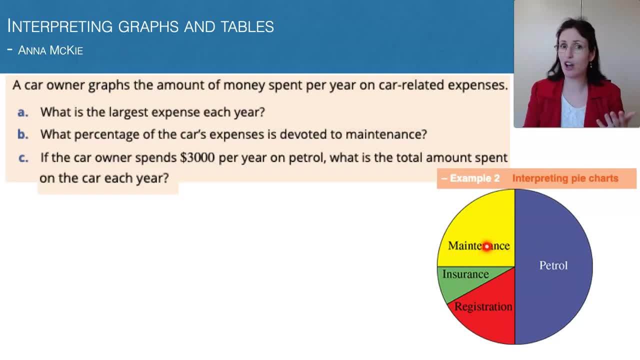 then we have maintenance here, which would be things like a service, maybe tires registration to make sure your car is registered, and insurance. so part a: what is the largest expense each year? which section fills up the most of the pie chart? petrol. so part a: what is the largest expense each year? we could write petrol. part b: 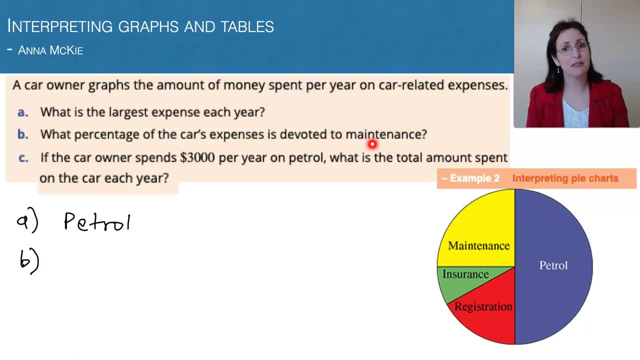 what percentage of the car's expenses is devoted to maintenance. so let's find maintenance and what percentage. so the whole pie graph would be: what percent- 100 percent- and petrol takes up half or 50 percent? and what fraction there do you think maintenance is? it looks like it's a quarter of. 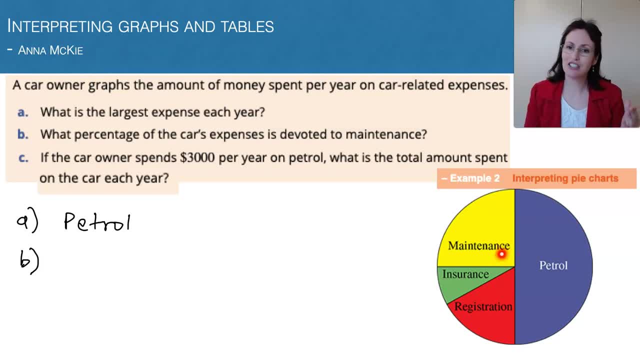 the pie chart and a quarter as a percentage, though it is one quarter of one hundred and that would be 25 percent. have we answered the question: what percentage of the car's expenses is devoted to maintenance? 25 percent, good and part c if the car owner spends three thousand dollars per year on. 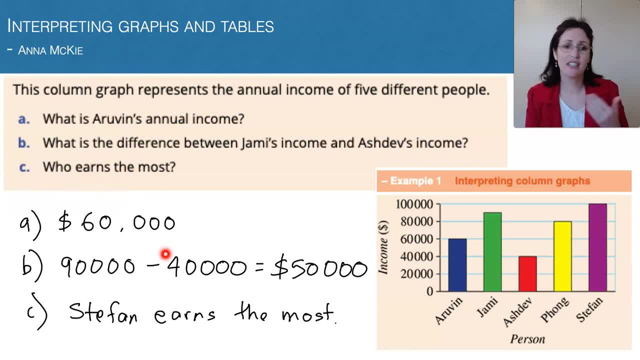 You can also calculate the number one of them here. what number does it fill? how many people? how many people and who are paying the Tooonds сил in this column? it's a good technique that when you're asked a question in a sentence, it's a good technique to. 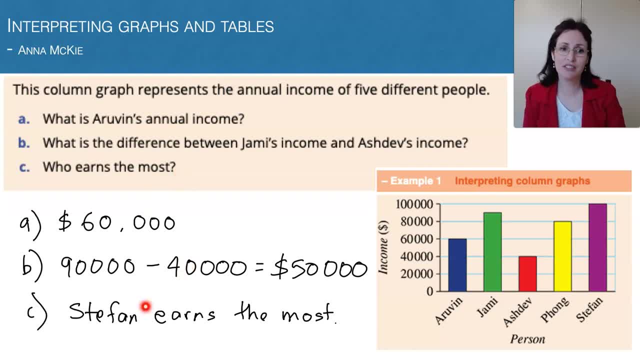 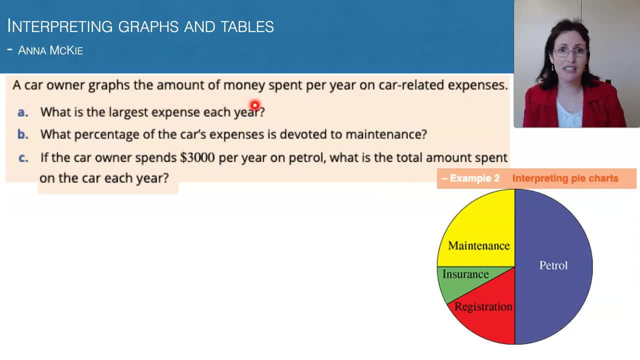 practice writing the answer in a sentence. who earns the most? stefan earns the most. second question: a car owner graphs the amount of money spent per year on car related expenses. so let's have a look here of our pie chart. these are all the different costs that you might spend. 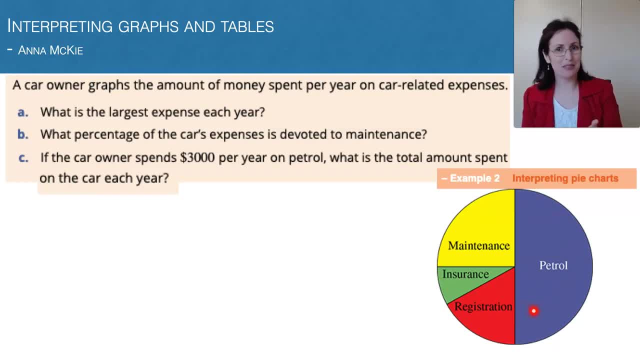 um, if you own a car about, um, that much is petrol, how much of the graph would you say? that is half or fifty percent. then we have maintenance here, which would be things like a service, maybe tires registration to make sure your car's registered, and insurance. so, part a, what is? 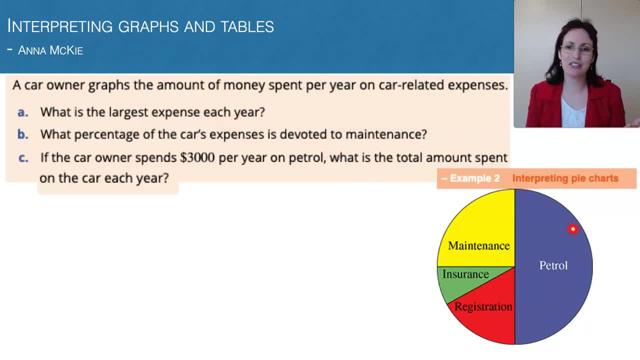 the largest expense each year. which section fills up the most of the pie chart? petrol. so part a: what is the largest expense each year? we could write petrol. part b: what percentage of the car's expenses is devoted to maintenance? so let's find maintenance and what percentage. so the whole pie graph would be what percent? 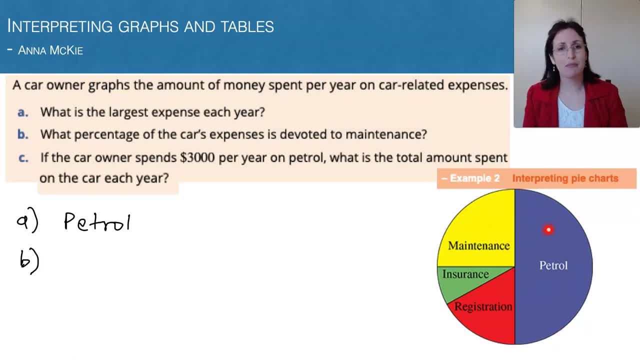 100 and petrol takes up half or 50. and what fraction there do you think maintenance is? it looks like it's a quarter of the pie chart and a quarter as a percentage, though it is one quarter of 100 and that would be 25 percent. have we answered the question? what percentage of the car's? 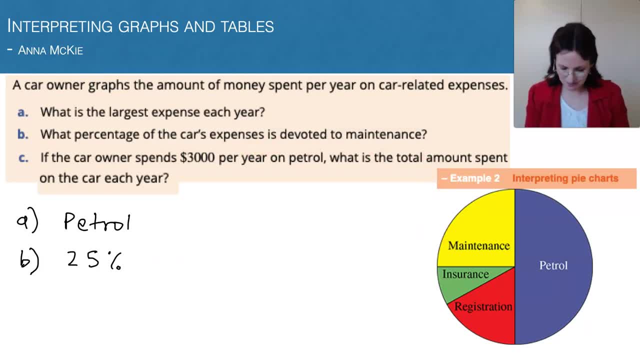 is devoted to maintenance. 25 good and part c. if the car owner spends three thousand dollars per year on petrol, what is the total amount spent on the car each year? so if that portion of the graph is three thousand, what would this portion be to make up the total amount? i'm sure you can. 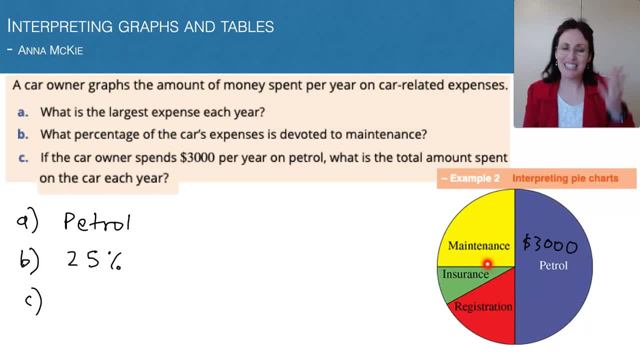 already anticipate that, but how would you write that out? basically, as math teachers, we want to see what's going on in your brain. we want to see how you think. so one way you might think of that is: well, 50 is three thousand dollars and we're interested in 100 of the graph. well, how do you? 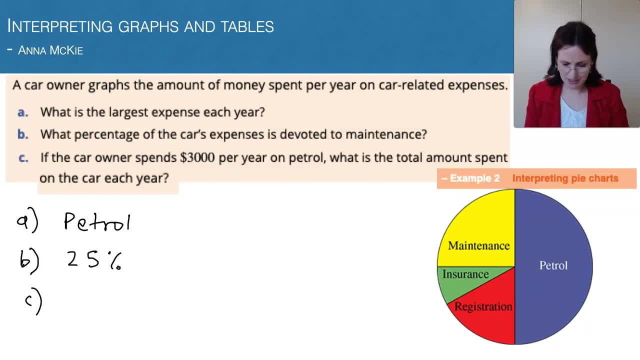 petrol. what is the total amount spent on the car each year? so if that portion of the graph is 3000, what would this portion be to make up the total amount? Do you havechine currently the almighty? do you haveśnie louis is carrying two pounds. i'm sure you already anticipate that, but how would you write that out? 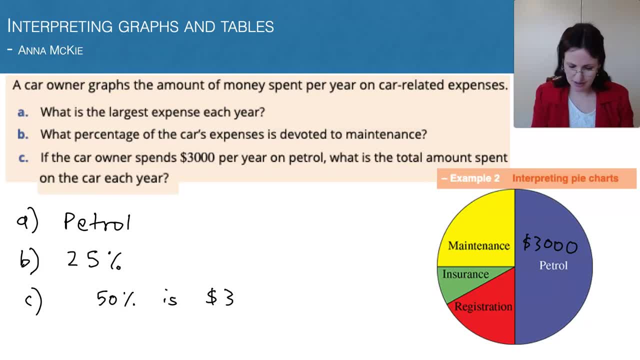 basically, as math teachers, we want to see what's going on in your brain. we want to see how you think. so one way you might think of that is: well, 50 is 3 000 and we're interested in 100 of the graph. well, how do you turn 50 into 100? what operation would you have to do to that? you would 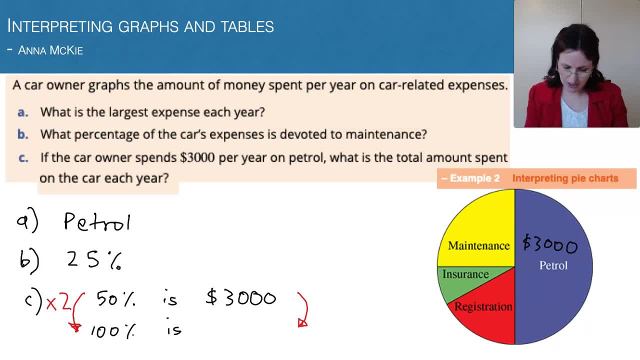 multiply by two, which means then you get k by dimensional square considered in the normal world. you have to take the $3,000 and multiply that by two as well to give you a number of $6,000.. So the question: what's the total amount spent on the car each year? $6,000.. We should write. 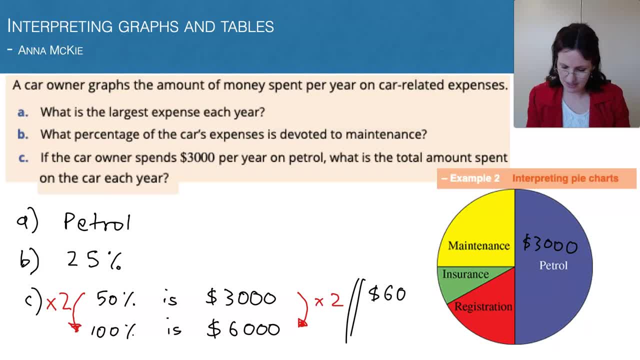 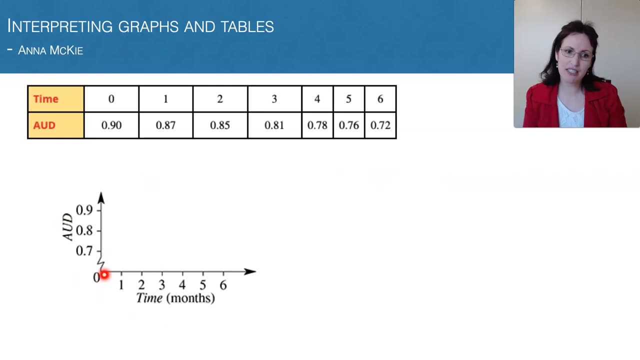 that as a sentence Running out of room there, $6,000 is the total amount. That's that question. And last one, not a question so much, but just something to be aware of. Looking at this graph here, you might notice something different on this vertical axis. 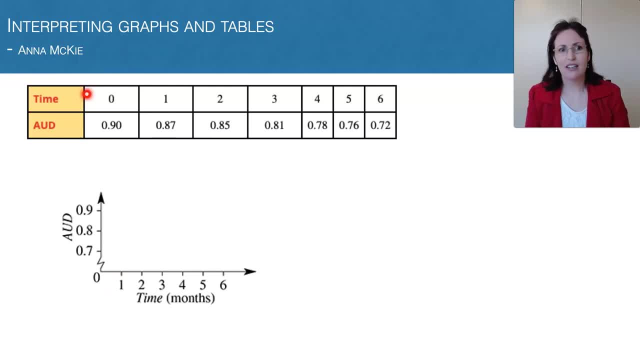 We call that a broken scale. Have a think about why. If you had to graph these numbers, noticing that most of these numbers are between the 0.7, 0.8, 0.9.. So if you were to draw a graph, 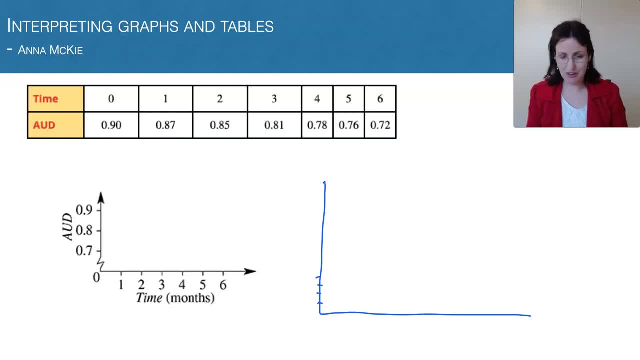 and these were going up by 0.1s. you would have 0.1,, 0.2,, 0.3,, 0.4,, 0.5,, 0.6,, 0.7,, 0.8, and 0.9.. 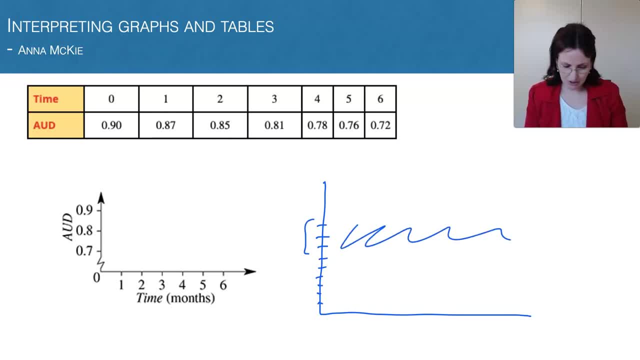 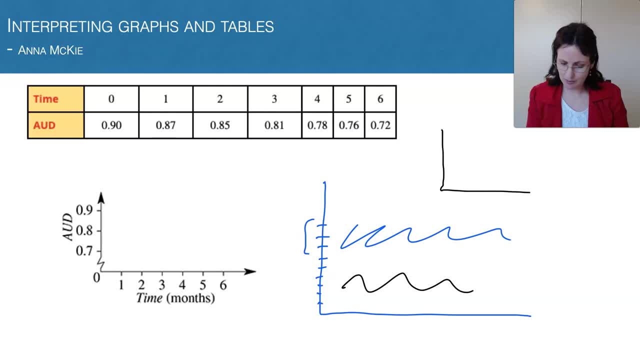 We don't really want most of what's happening down here, So we sometimes put what could be called train tracks in. that's showing that you've broken the scale. Or sometimes it's a squiggly line as you're drawing the graph, to show that you're the reader, that you know that there's actually. 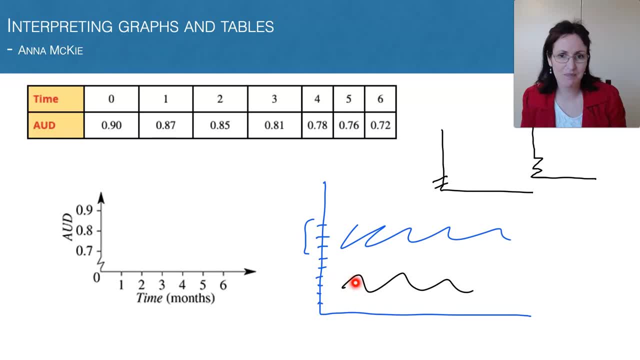 numbers that are in here, but we don't need to show them for now. Okay, so that video is on interpreting graphs and tables.